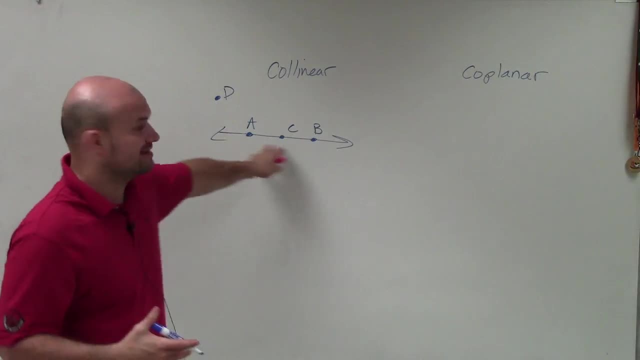 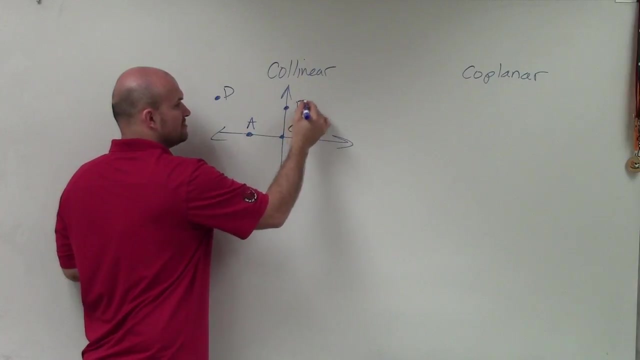 So therefore point D is non-collinear or not collinear. with these other points I can also draw another intersecting line And let's call this point E, So you can say that Still A, C and B, those are all collinear points, right. 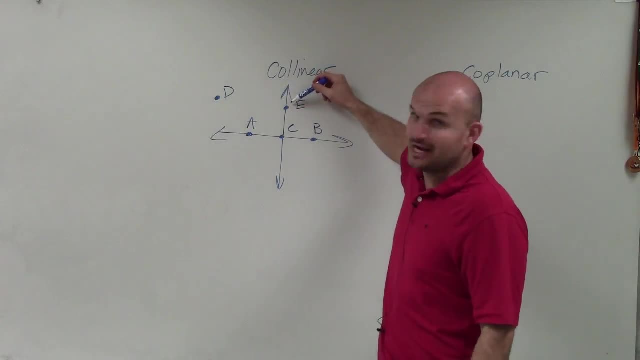 They all lie on the same line. However, point E is not collinear, does not lie on the same line. It lies on the same line with E and C. We could say those are collinear. but it is not collinear with A, C and B. 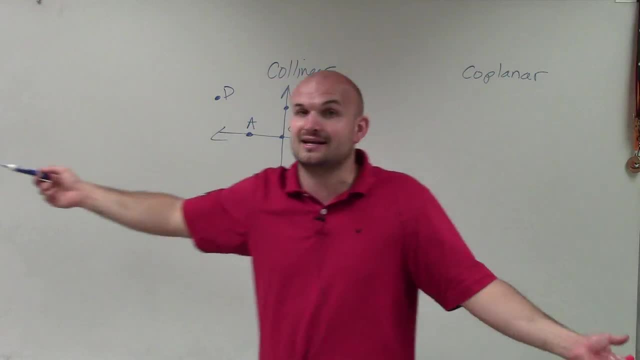 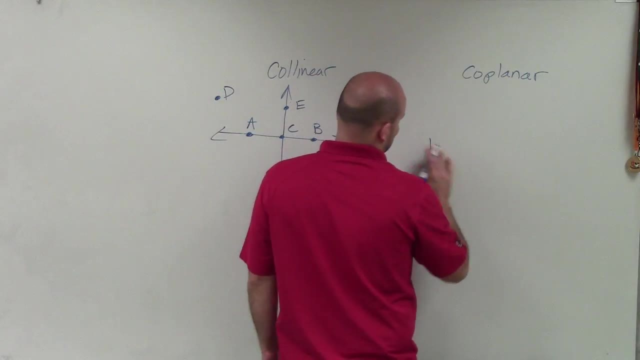 as well as the same thing with D, because that's not on any line. So obviously it's not on the same line When we're looking at coplanar- and I like getting with coplanar because it's always very difficult to understand. 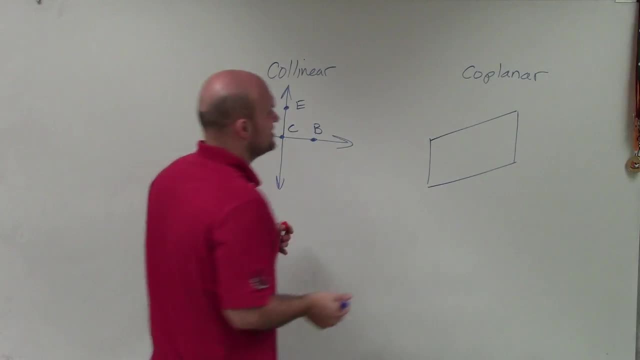 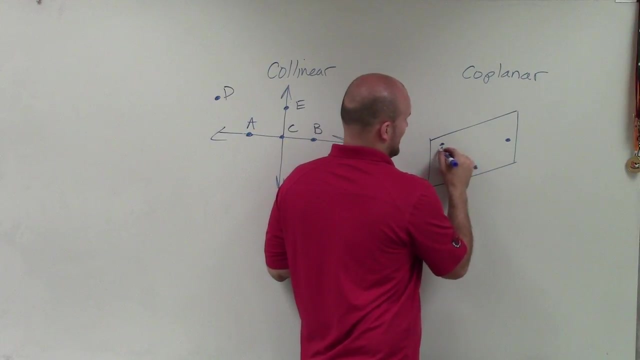 kind of graphing a flat surface that extends indefinitely. So coplanar is just going to be any points again that lie on the same line. So let's call this A, B and C. I'm sorry, not lie on the same line. lie on the same plane. 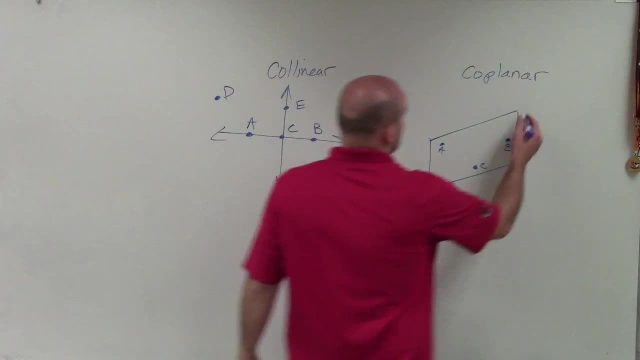 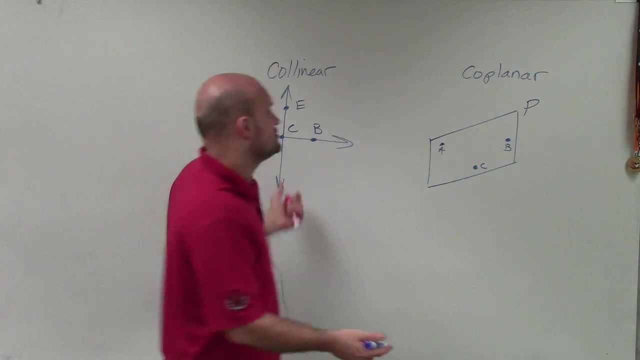 So since these points all lie on the same plane, let's call this plane P, then they are coplanar, right, Just like collinear. they lie on the same plane, so they're coplanar. So then obviously, if I kind of 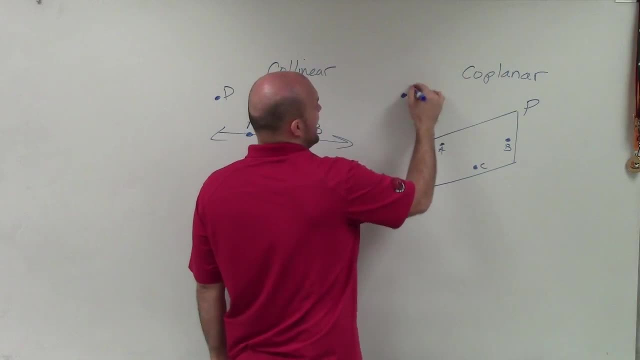 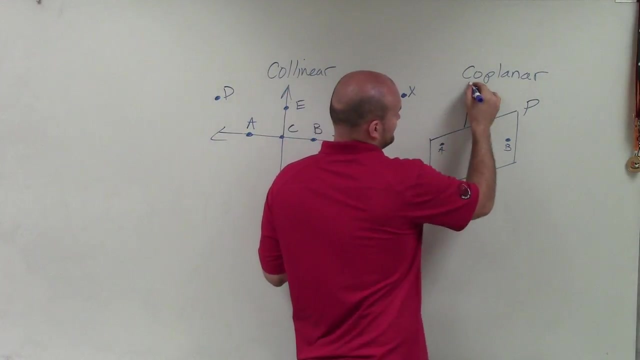 If I have a point that's off of this, let's call this X. you can see that X is non-coplanar or not coplanar with the other points. I'm going to try to do my best here. And what if we had another plane? 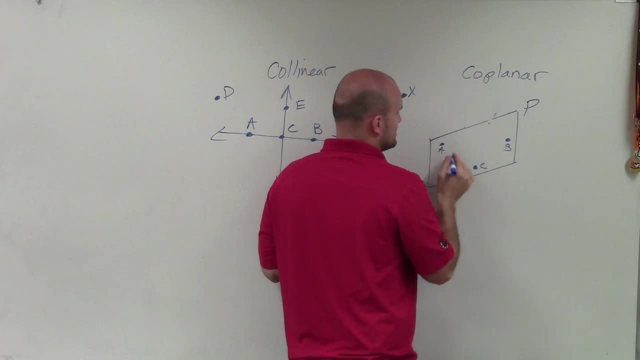 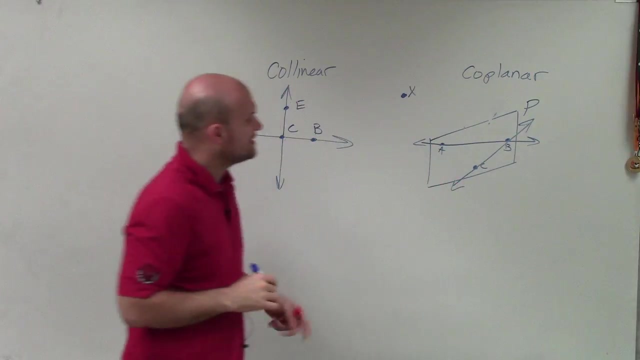 Actually hold on before I even get to that point. I forgot to mention as far as lines, So I could also have coplanar lines. So you can see that the lines A, B and the line C both all lie on the plane. 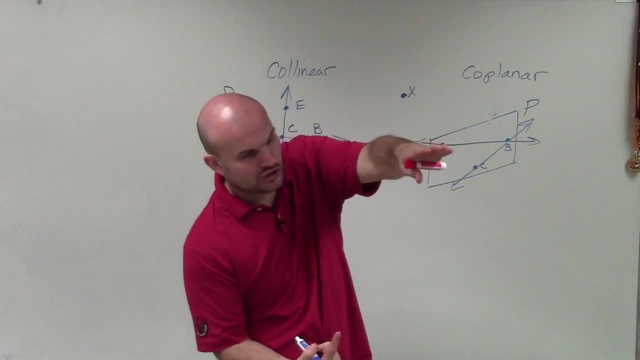 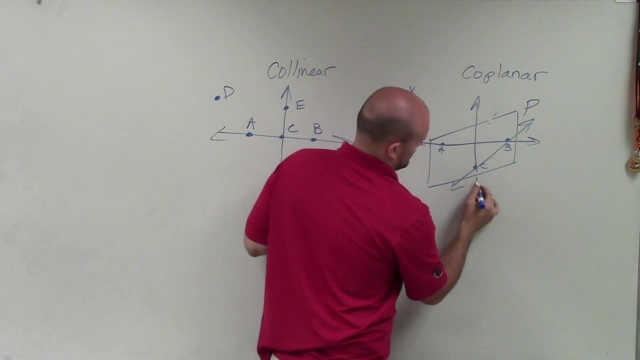 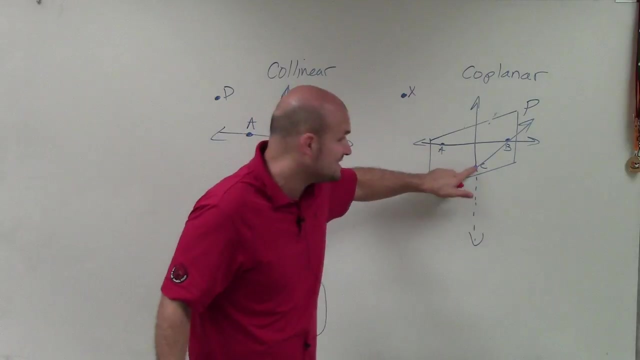 However, if I was going to you know, think about if we have a flat surface- and I was to shoot a line going straight up, which I'll try to represent like this. So this line is going perpendicular from the plane. Therefore, the point still lies on the plane.